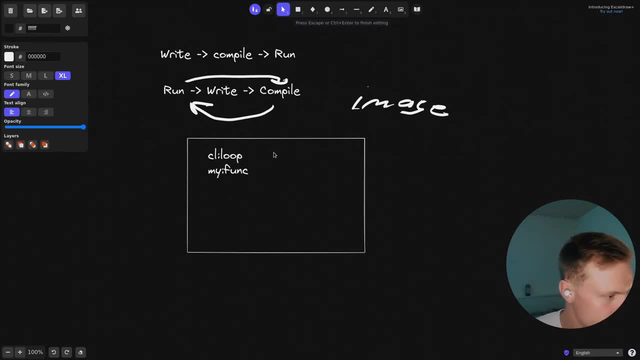 and you'd also have your own stuff, like my, So this, and you'd have like all the CL namespace stuff. So you'd have like if and all that sort of stuff, all the stuff that comes with common Lisp. So when you first start, 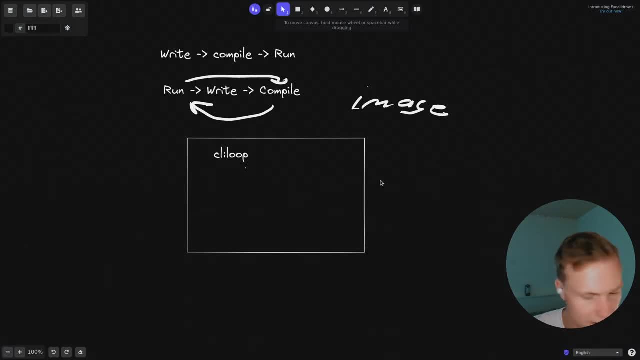 Lisp image, you end up with just a blank image and you add different symbols to it. And so when you're writing code, so say, I write a program and I write a little function and I compile it with slime or something like that. So what I'm doing is I'm actually putting new code into my Lisp image. 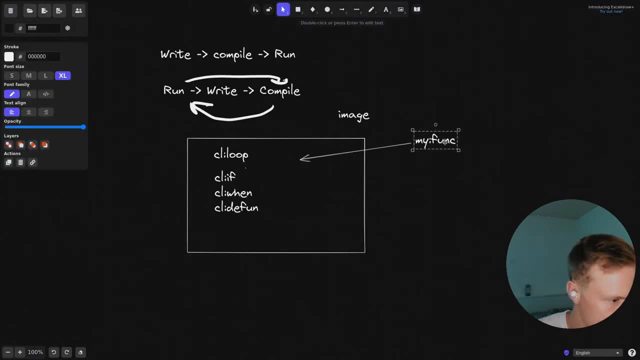 So now what we have here is we have basically the general stuff. So we've got our new function that we've put in and it's going into our Lisp image and there we go. So now we no longer need that arrow, We have our function in here, And so we've basically added code to our 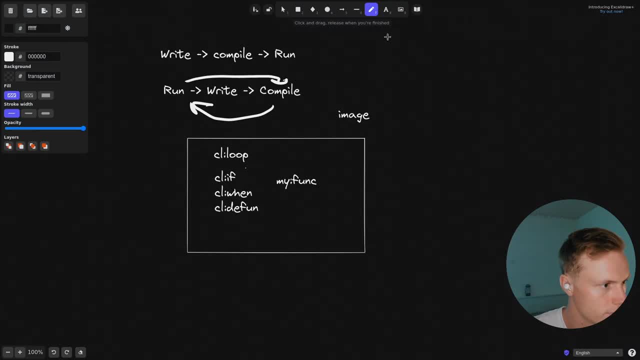 Lisp image and this code can actually run with our running image. Basically, what we've done is we've started up a REPL, we've added code to the REPL and we can execute it And that might sound kind of simple, but the idea is that basically, this Lisp image is constantly being updated. 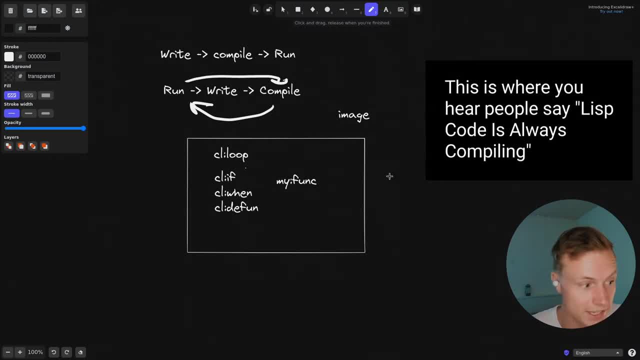 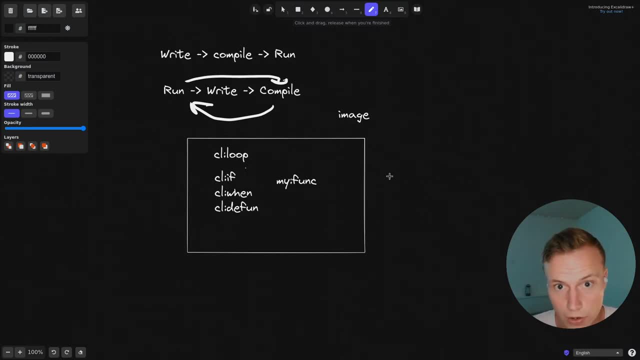 And then when we want to actually make a final executable, all we're basically doing is just dumping that image and then telling it what, what a symbol to start calling when we give it our program. So when we want to execute code, that's all we're doing is we're just calling a function. 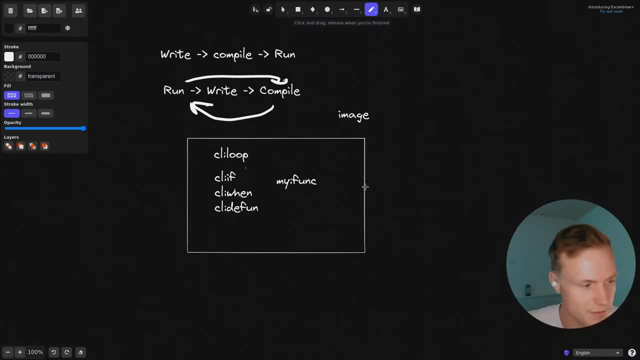 and so this is kind of why the common Lisp build system is a bit strange. You aren't just making a single binary, You have to give it all this extra information, And that's basically because you're just taking kind of what you can accumulatively think of as kind of a operating 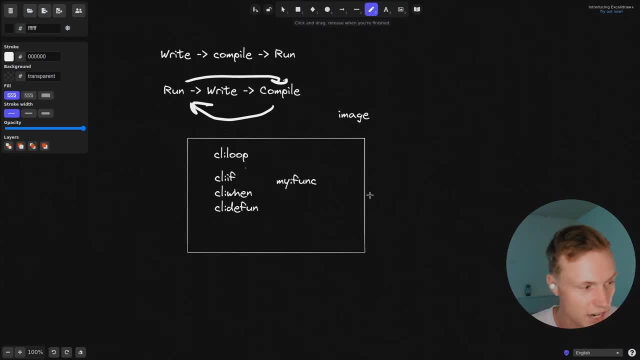 system image. If you've ever installed a Linux distribution, it's kind of a similar idea. You're basically creating a state that the program will run in when you execute it and then giving that to the user And that's what you're getting. with a disk image, What actual kind of benefits do you? 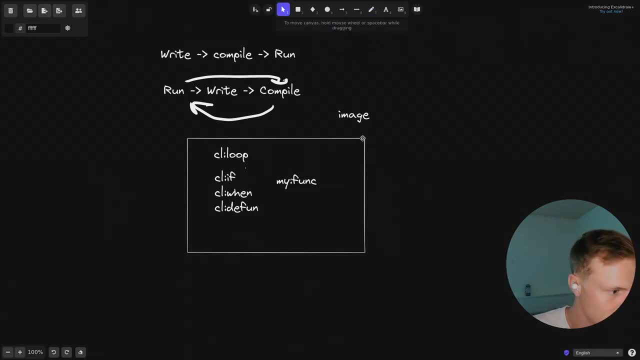 get out of this. Well, the biggest benefit is that you don't have to worry about the actual state when you build. it is going to be pretty much identical to the state when you actually run it. So as an advantage, you basically- let's just move this over here. So when 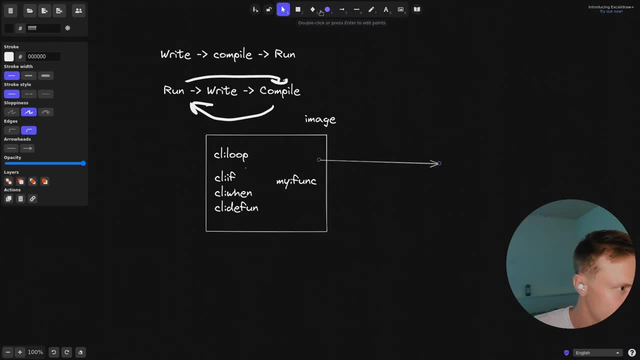 we get our final executable right here. you can actually make it possible to update it So you get that same Lisp image as before. but you can actually add your own code and change things. So for example say, we copy this guy and we put him here, And so here we have a Lisp image that's. 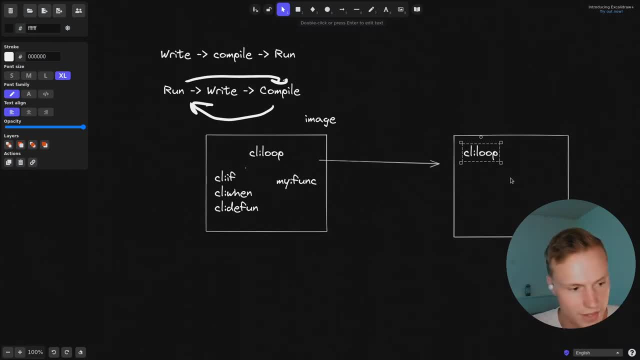 going to be the same as before, So we can actually do that. So let's say, we have all the same stuff, but maybe we want to redefine loop and we can do that while we have the executable, And so this might sound a bit obtuse and why would you even use this? But this is really powerful for debugging. 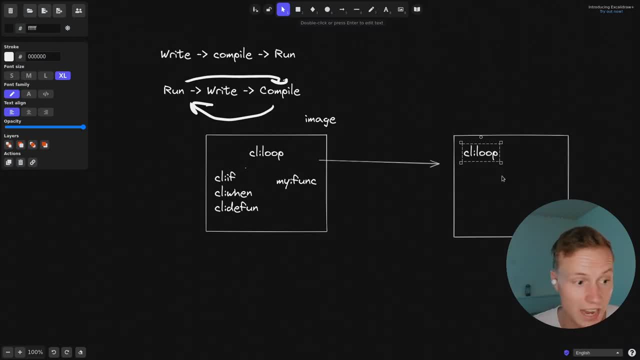 If you guys have ever had a server that's run into issues and you want to see what's happening, you can actually interact with it live just via a simple REPL. And let's give you guys a really good example of this using the Nix browser, which is written in Common Lisp. Yeah, let's go ahead and pull that open. 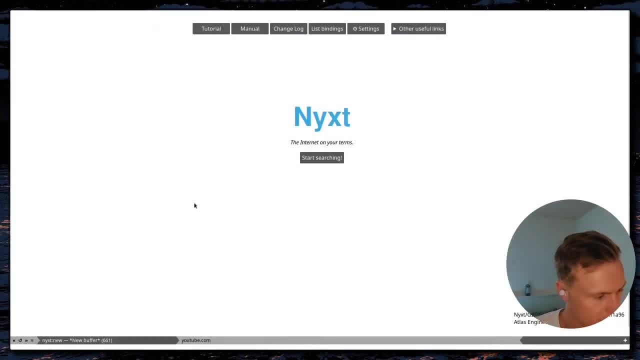 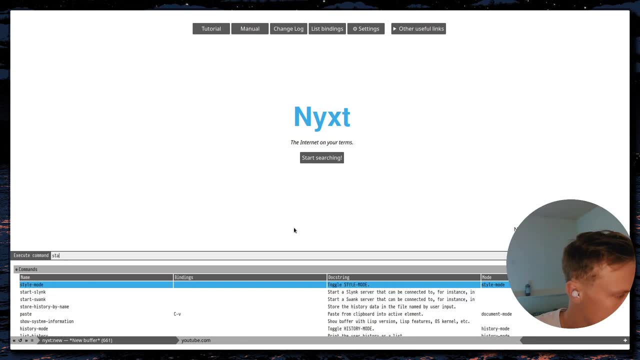 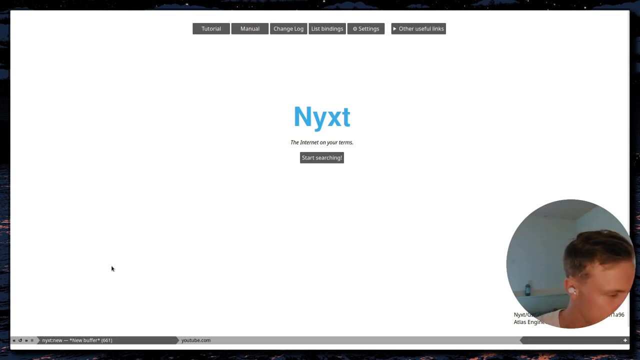 So, switching over to the Nix browser, you'll see a few things. There's just a little browser right in front of us And if we want to run a command, the first thing we'll want to do is run this command called start slink. Now this will run. you'll see right down here running on port 4006.. 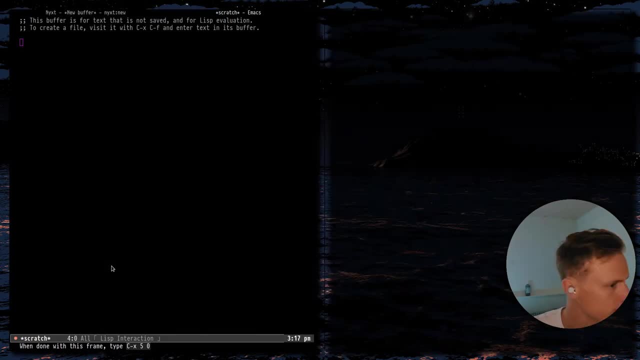 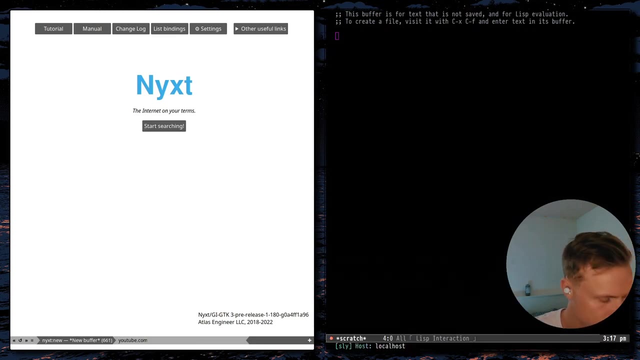 So I'll just open up Emacs just for this video And in Emacs I will run sly connect All right, now that we have this REPL running and we are connected to that running lisp image, we can actually manipulate it. So, for example, if we wanted to- I don't know, let's see what another command is- Let's do like watch. 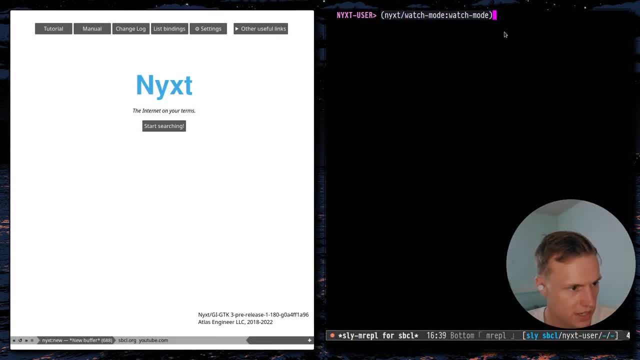 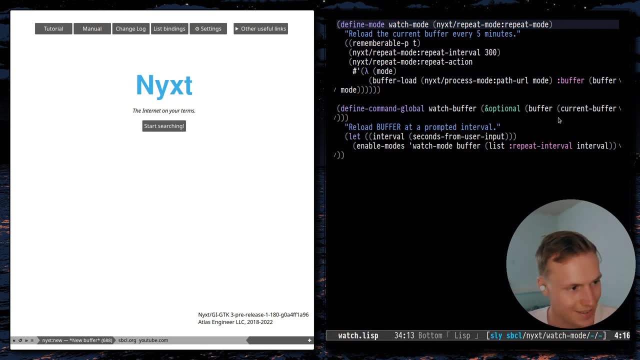 mode. We get access to it right here, as you guys can see, And we can even go to the definition. Yeah, And we can go to the definition. We can. obviously you can see the documentation right there, but if we wanted to, we could see the documentation. It gives you a lot of information. 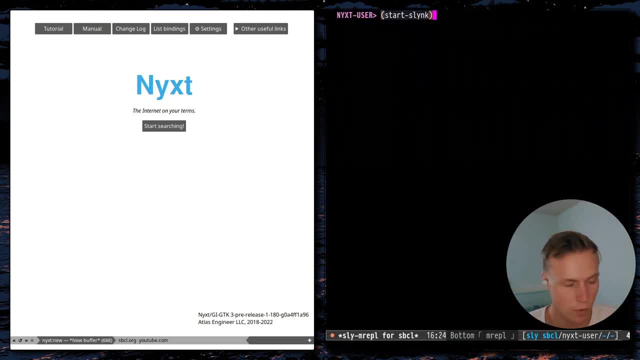 But anyways, that's not what we'll be working on today. So, like I said, said before, you get a lot of an advantage out of this um, out of this program that we have here, because we can actually manipulate it, since it's a lisp image, and so because of that, you can actually 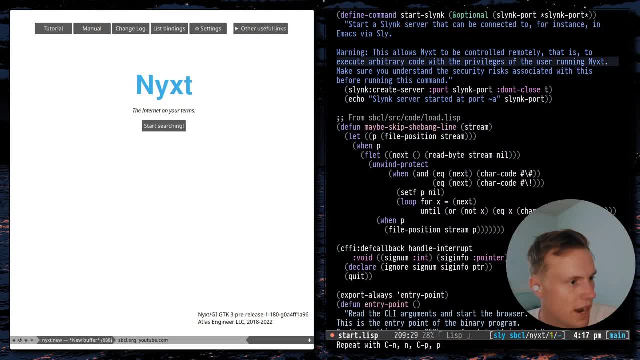 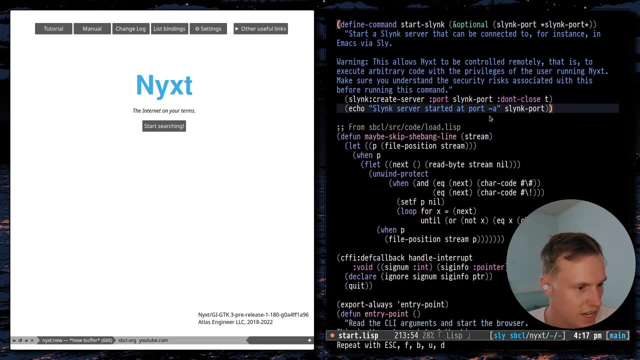 look at the original source code. um, there we go. i have the original source code for the starts link right here. i just jumped to the definition right before switching um and we get a lot of information and we can even evaluate code that will active- uh, be active in the browser. comment this out. 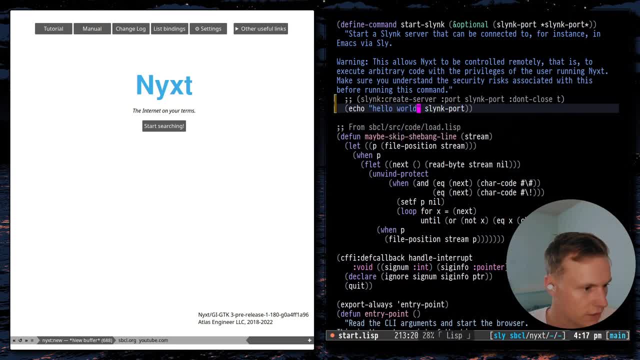 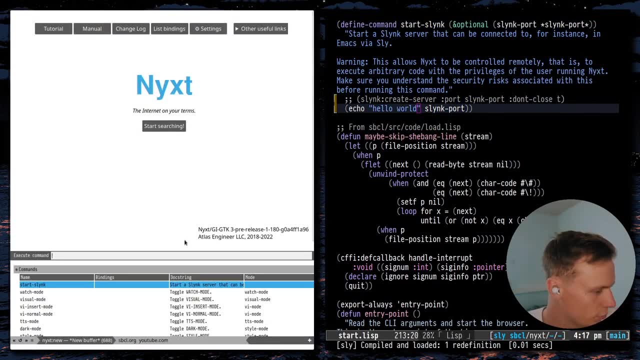 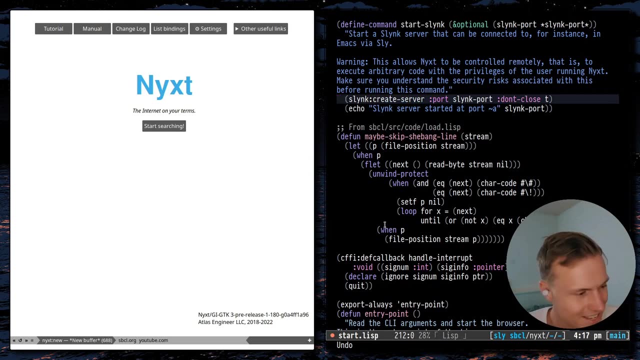 and make it just echo hello world. all right, everyone's favorite thing to do. now i could compile that and then in next, if i just run starts link, it will print hello world. so there you go. there's the proof that we are actually editing the current instance, and so a common thing that 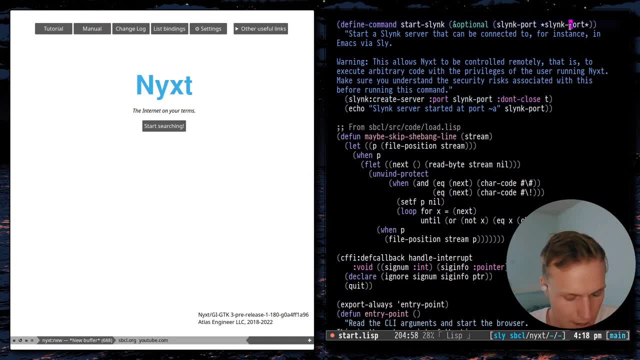 you will notice is that you'll sometimes want to be able to change things. so, for example, if i were to evaluate this, we'll see that this is a set port number. we can actually change it to a set port number, and we can actually change it to a set port number, and we can actually. 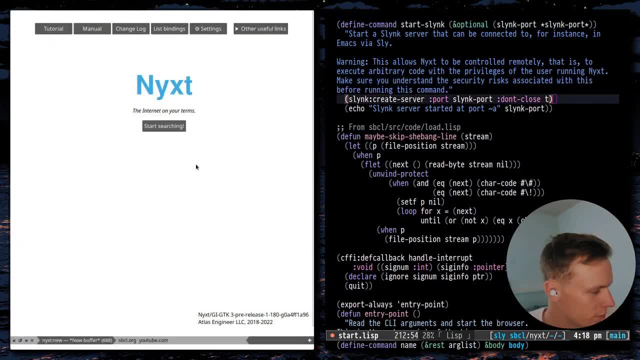 um, when we run it, so that's not particularly helpful, and so if we were to run it again, i assume we'll get an error. oh sorry, i gotta recompile it. and so now, if we run it again, starts link. yeah, we get an error because the address is already in use. so what, we're going. 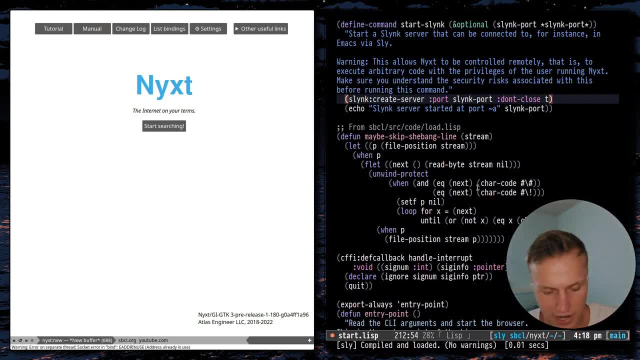 to go ahead and do? is we're going to actually manipulate this to make it better and make it so that way it can handle errors like this? uh, because, while in this case the port is in use because we're actually connected to a repl, port 4006 can be in use for really any reason, and 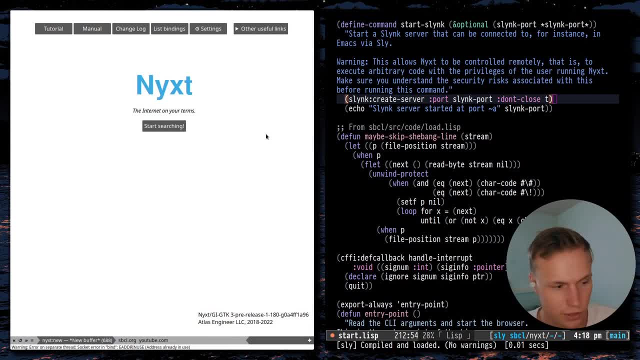 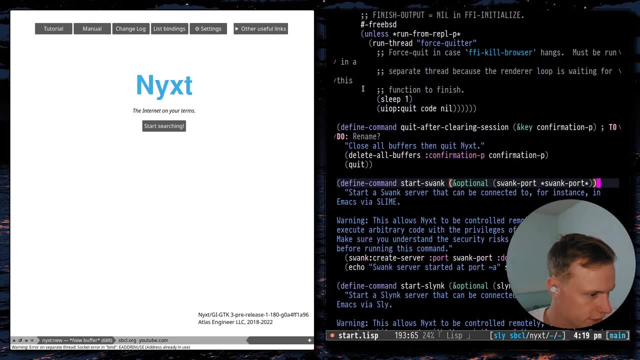 it would be nice to make it so. that way the user can change this, uh, without having to do anything to manually manipulate the code. and so, for this case, what we'll want to do is we will want to let's just recenter this. so there we go. so we've just narrowed it to the current function. now what? 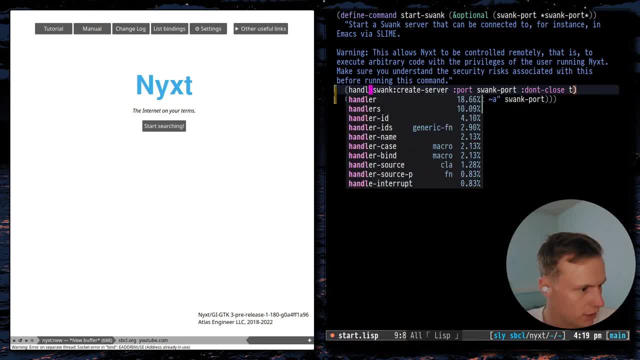 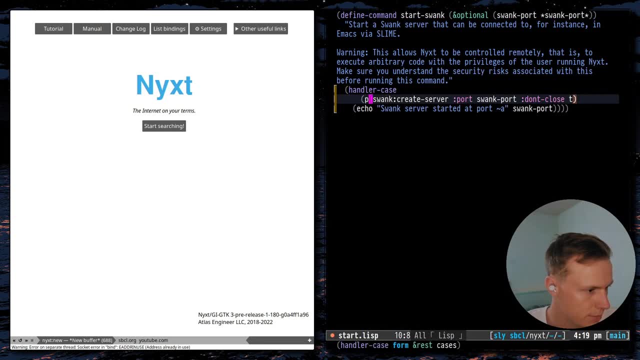 we're going to go ahead and do is actually handle this. so we're going to want to write a handler case and this is basically how you handle errors, and we'll just wrap this guy a progen just that way. when it handles an error, it will skip over both these guys. 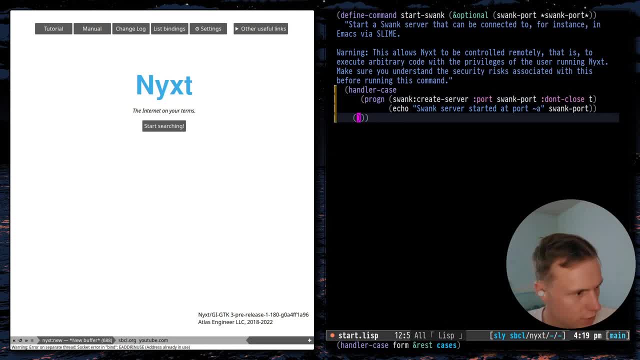 and then for the kind of error that we want to handle, we're going to do in, what did it say to do socket bind address already in use? um, here we'll just go ahead and, uh, what do we want to do? we'll just do error, so we'll just catch all errors. 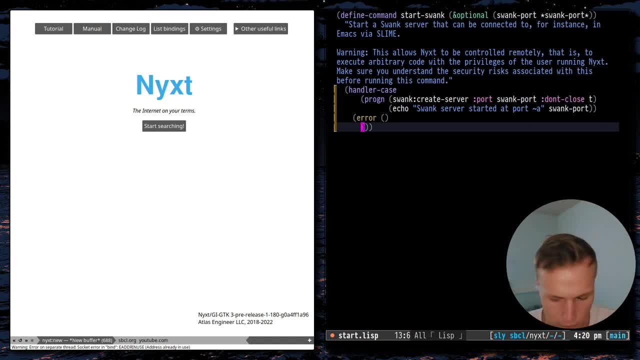 we don't really care what kind of error it was, and then we will have to do something with it, and then next up we'll want a way to handle this error. um, so i've actually written this part ahead of time, uh, just to kind of save us some time in this video. there we go, so now, what we're doing now. 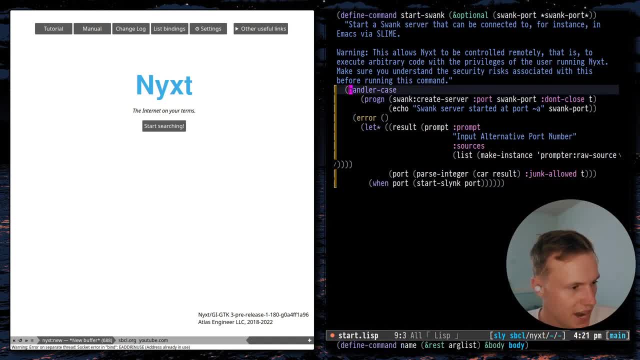 basically, this looks actually very similar to the original, but all we're doing is we're adding this handle case which will basically catch any error, which, in this case, will be when the port is already in use, um, and then what we will do is we'll bind the result. and so when i say 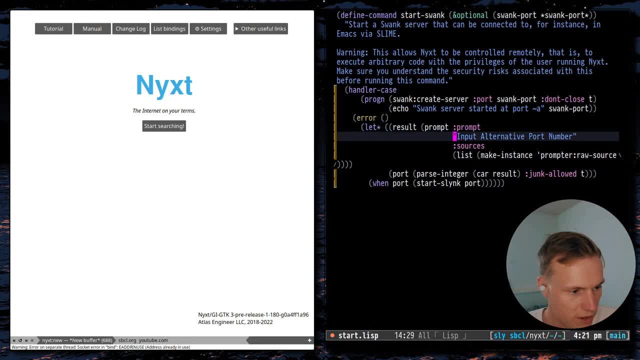 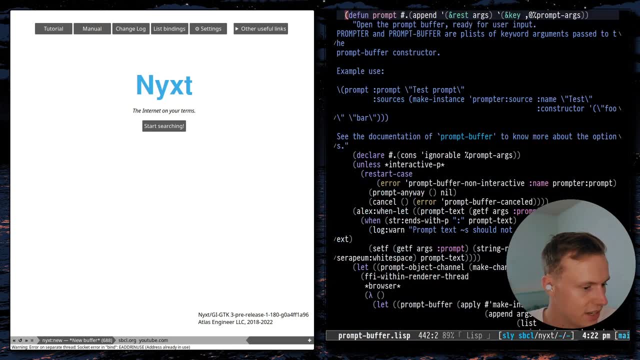 result. in this case that will just be, uh, the port number, and it'll prompt for this port number using the prompt function. this is actually part of next. i can just go ahead and jump to the definition. pretty neat. so basically, how this will be done is: we'll basically call this function, we'll get 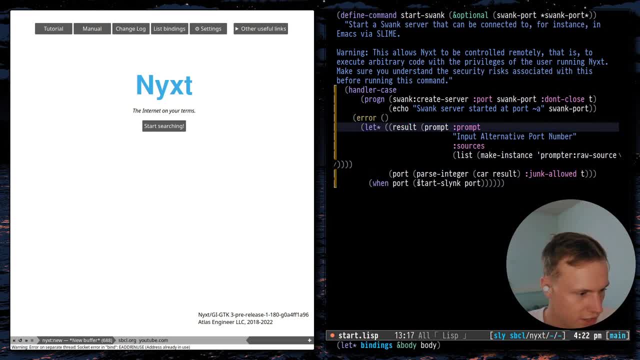 the result and store it in result, and then we will press it as an integer and then, when we have a port number, we will go ahead and start slink again. so let's go ahead and compile that, and then in next we will go ahead and run start slink. oh, my solution did not work one sec. 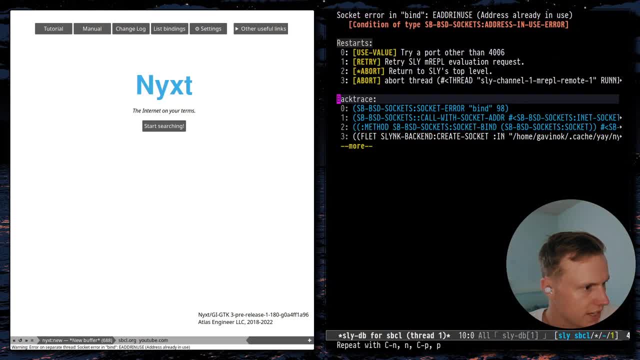 so, just in case, i'm just going to go ahead and run, start slink again and catch the. it doesn't actually say error in here, oh no, it says error there. i don't know, this might not be necessary. we'll go back to the code again and we will just replace the error with this. 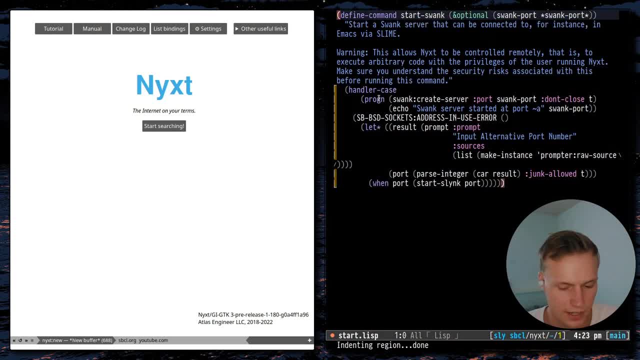 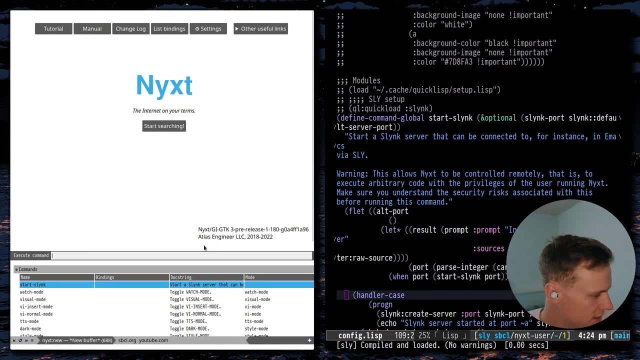 and this will basically say exactly what kind of error this is. technically it's a condition, but we won't get too technical for this, um, and so now in here and run start slink. there we go. now we will be prompted for the user input and we'll just do 4002, hit enter and then it will start the port on. 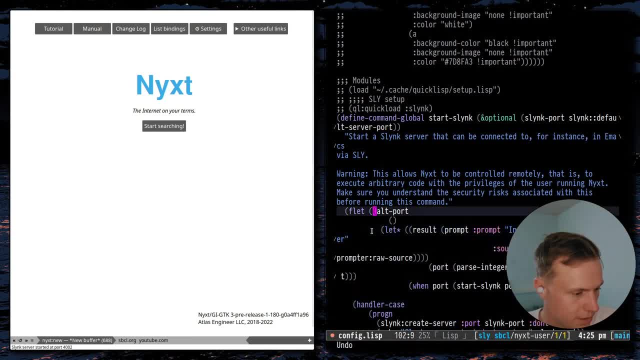 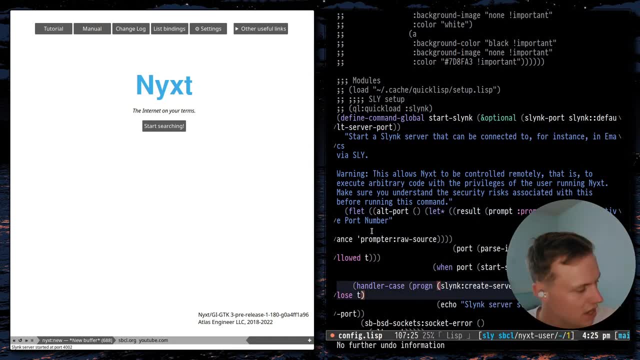 4002.. um, pretty cool, and all we did was actually manipulate the original code. if we go back to the original, we can always go back to the original, and if we were to restart next, it will just use the original code. but if we were to add this to like, say, for example, our configuration: 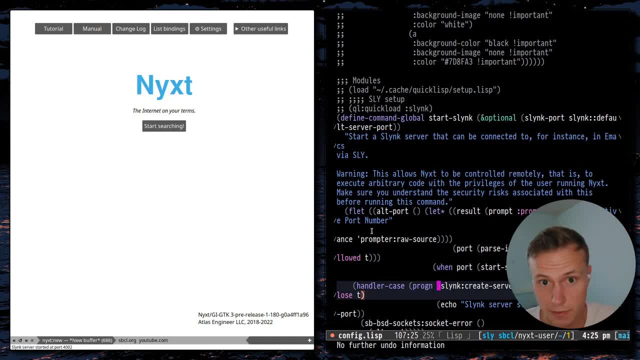 or anything like that. then we can actually load that code into the lisp image. and this is kind of how lisp in general works. we're compiling code, that's all we're doing. we're taking a lisp image, putting in new functions and symbols, and then we're basically dumping an. 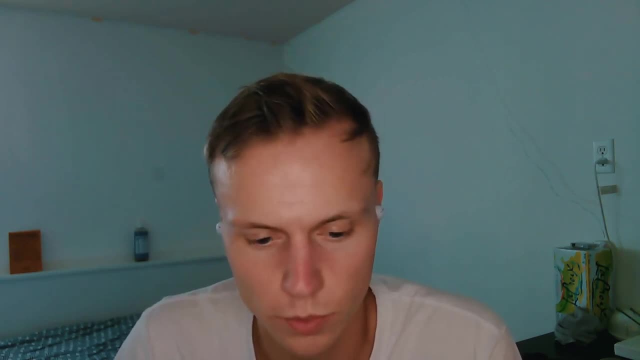 image of it. anyways, guys, that's all for today's video. i just wanted to kind of show off the power that you get from a lisp image, as well as the kind of advantages you get. what i just did with nixed is something you can't do with pretty much any other browser. could you imagine trying to?